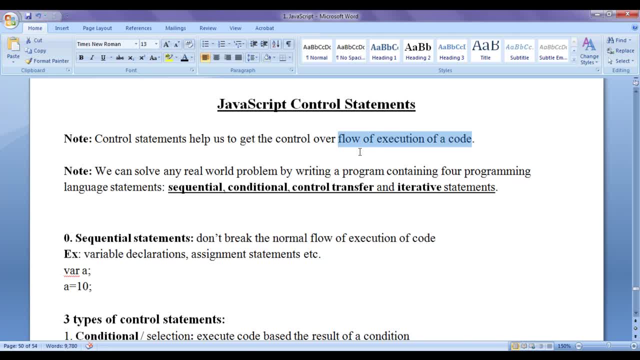 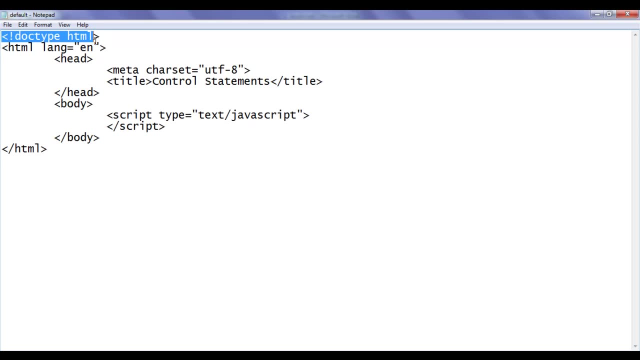 If we want to get the control over flow of execution of a code, we take help of JavaScript control statements. Let me explain clearly. I go to notepad. You can see that I have already opened defaulthtml in the notepad. It has the basic HTML document structure code. written Title is set to control statements. 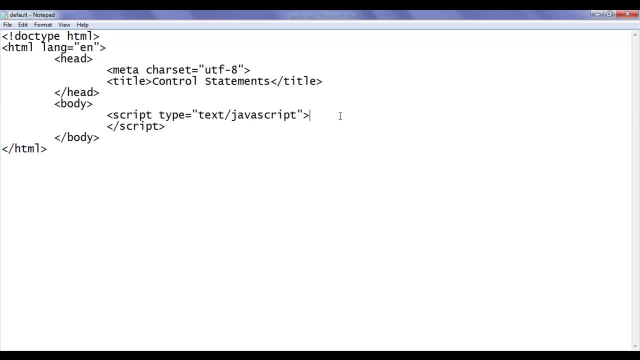 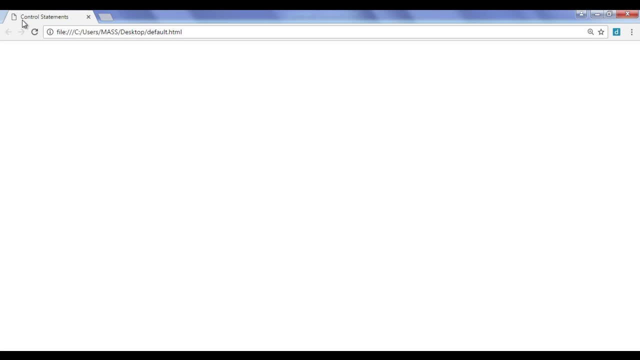 In the body section I have already written OpeningScript and ClosingScript tag. I have already opened. defaulthtml in the chrome Title is set to control statements. Let me go to notepad. In the taskbar I click on the Multi- contracting Stay title. In the taskbar field. let me display the defaulthtml. Default html in the chrome Title is set to control statements. Let me go to notepad. I click on operations and changes. the defaulthtml nosob is piloted mobile setting menu. The defaulthtml is currently pasting. 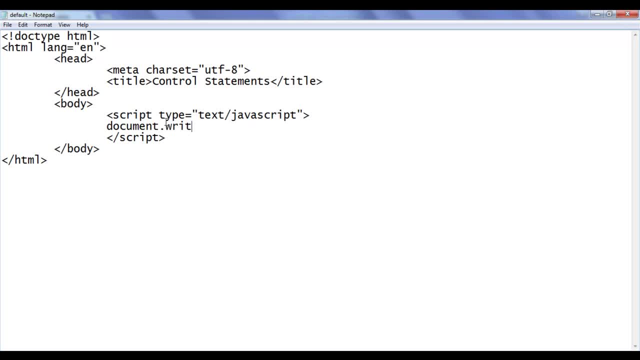 In between the script tag. I say here documentwrite in double quotations. I say hello world, one double quotations comma. I give here break tag semicolon. I copy this line of code: paste down one, two, three, four, five times. 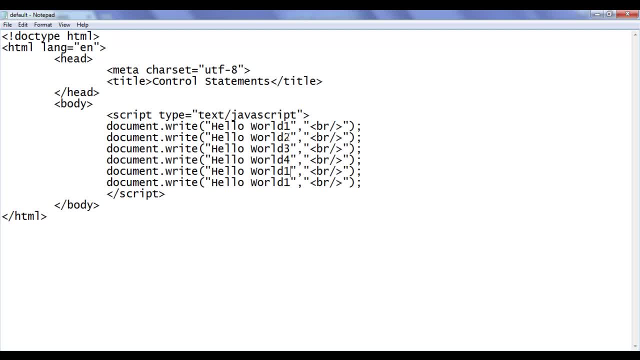 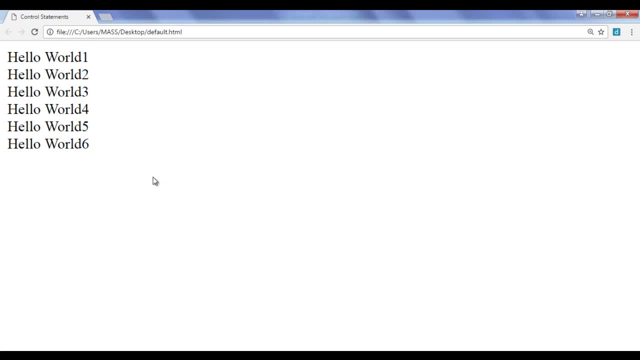 I say here: two, three, four, five, six, file save. go to browser and refresh. You can see that we got the output. hello world one. hello world two. hello world three. hello world four. hello world five. hello world six. 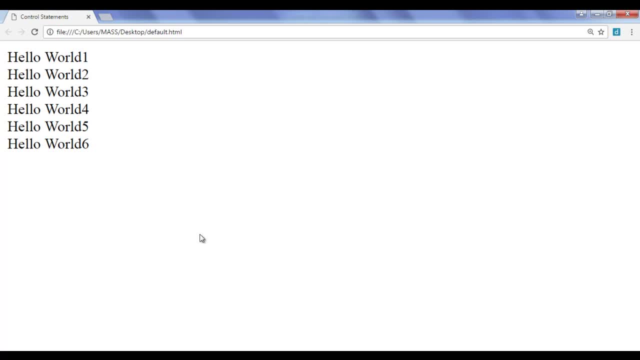 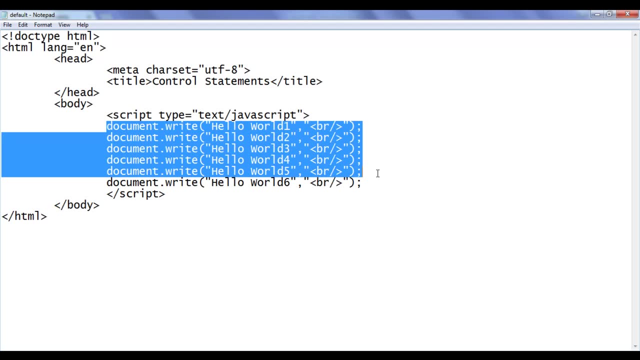 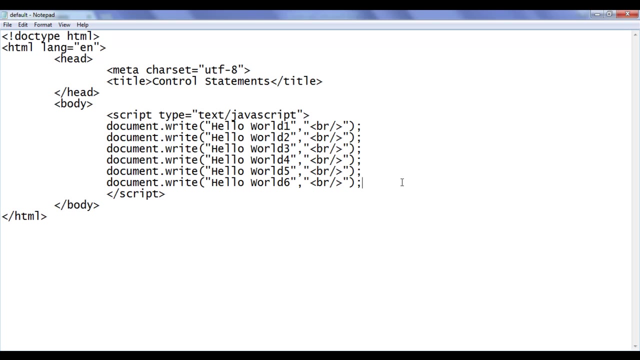 No statement is missing, right? What browser is doing here? Browser is executing each of these statements one after the another, sequentially, top to down, right? Remember that the normal flow of execution of code is sequential. Sequential means executing the statements one after the. 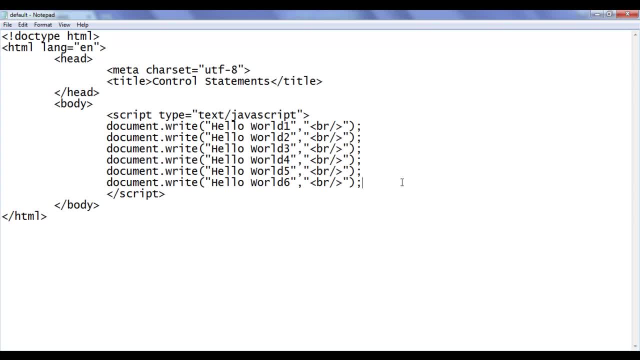 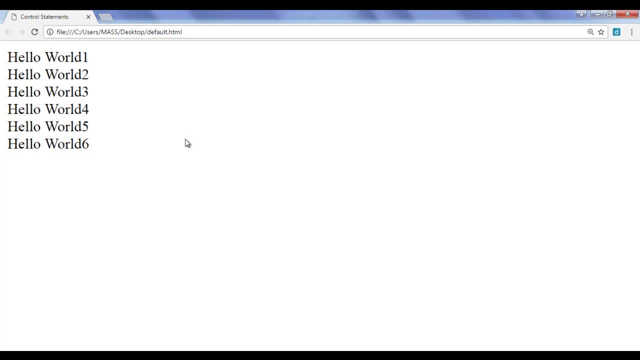 other sequentially, One after the other at a time, from top to down, without skipping any statements, right? That is the reason we are getting all the outputs. I don't want to get this output. I don't want to get hello world one. hello world. two. hello world. three: hello world. 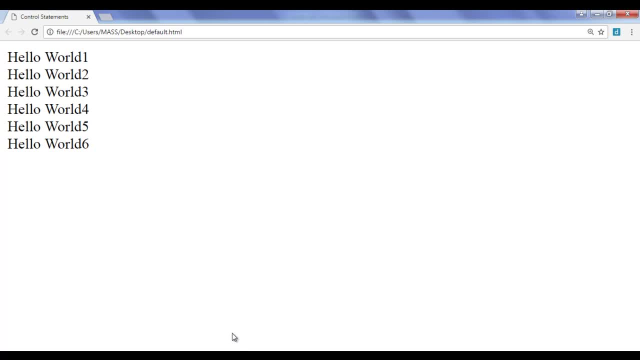 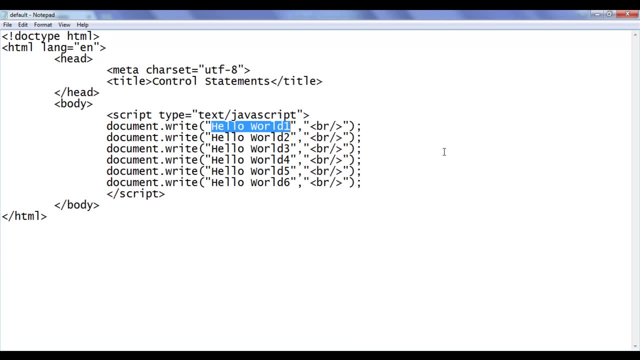 four: hello world five. hello world six. I want to tell to the browser something different. What I want is I want to tell to the browser: display hello world one. okay, The browser will display hello world one. then I tell to the browser: go directly to. 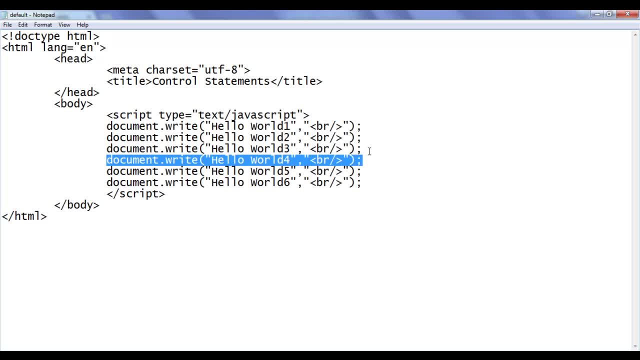 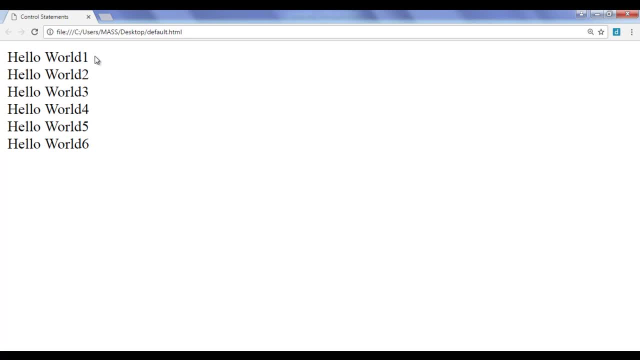 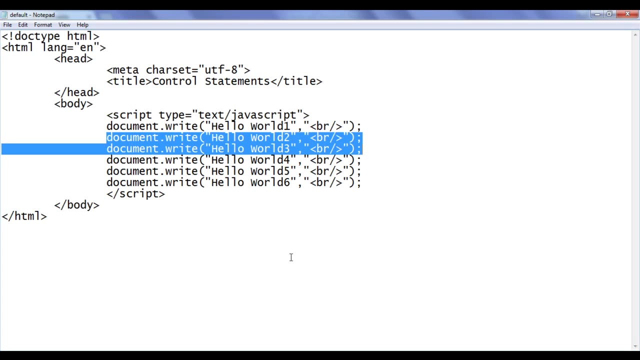 the fourth statement: display hello world four. You have to skip hello world two and hello world three. I don't want to see output hello world two and hello world three. You have to display hello world one and directly display hello world four. Now how do we do that? 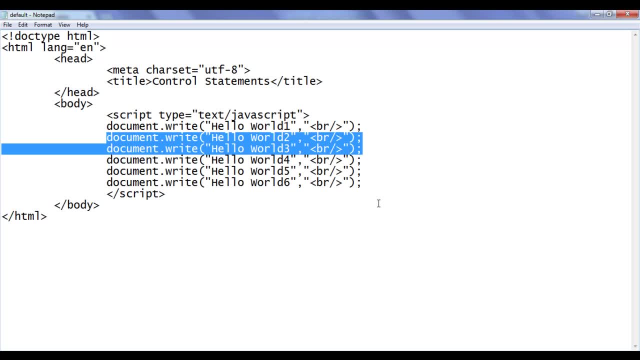 To skip a single statement or set of statements and transfer the control from one place to another place directly. JavaScript provides control Control transfer statements. Control transfer statements or jumping statements are used to skip a single statement or set of statements and jump or transfer or move the control from one place to another place. 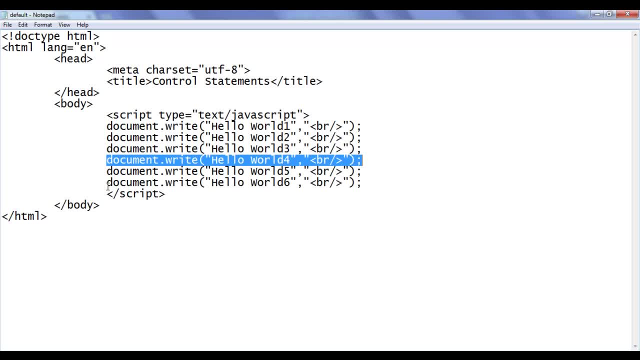 directly. Then I tell to the browser: before going to the sixth statement, you have to execute this fifth statement hundred times. Display hello world five one hundred times. Okay, Then display hello world six. I need more control here, right? So browser has to stop the control in this line and execute the statement one hundred. 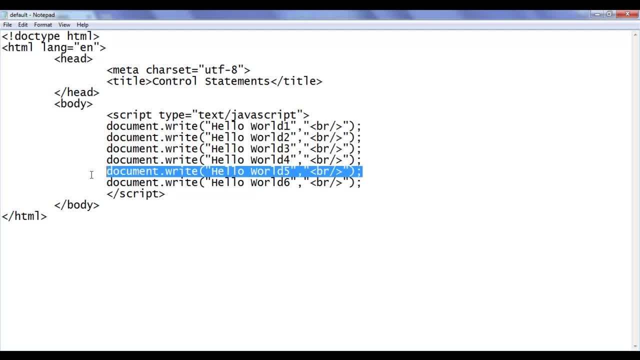 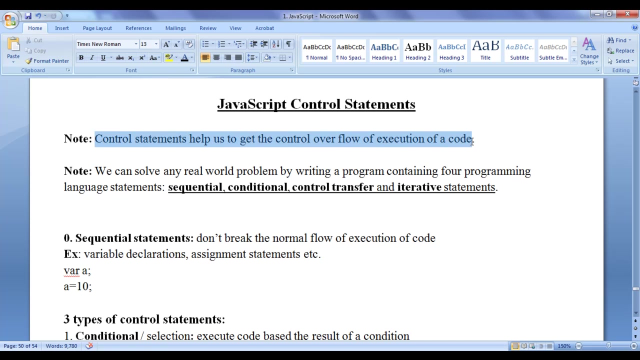 times repeatedly. That means to execute a single statement or set of statements repeatedly. JavaScript provides iterative or looping statements. We take help of iterative or looping control statements to execute a single statement or set of statements repeatedly. Hope you guys have clearly understood. Control statements help you to get the control over flow of execution of code. 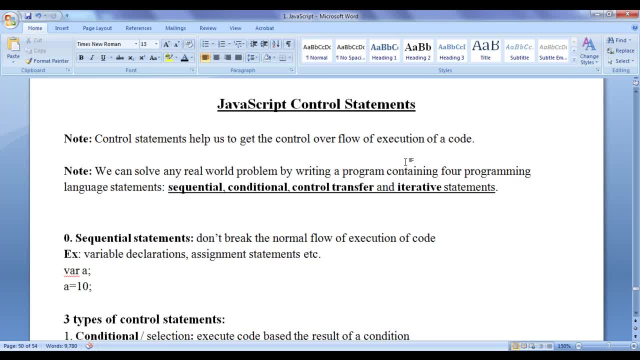 You can execute some set of statements according to your requirement. You can skip some statements. you can execute some statements repeatedly, right? One more note I want to give you here. We can solve any real world problem by writing a program containing four programming language. 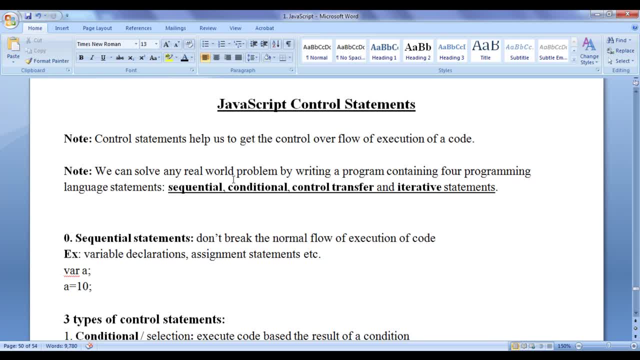 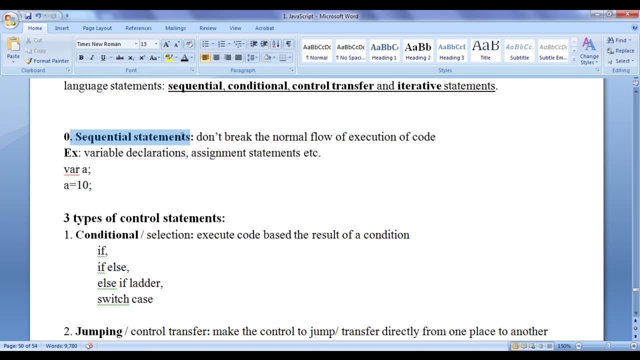 statements. These are sequential statements, conditional statements, control, transfer statements and iterative statements. We discuss each of these statements clearly. First. I talk about sequential statements. Sequential statements don't break the normal flow of execution of code. What is the normal flow of execution of code? 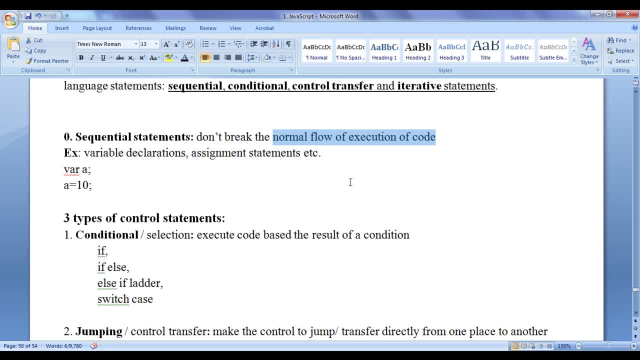 We know that the normal flow of execution code is sequential execution, Sequential execution, Executing the code top to down, one after the another, without skipping any statements. right Variable declarations and assignment statements are considered as sequential statements. For example, var a: this is a sequential statement. a equal to 10,: this is a sequential. 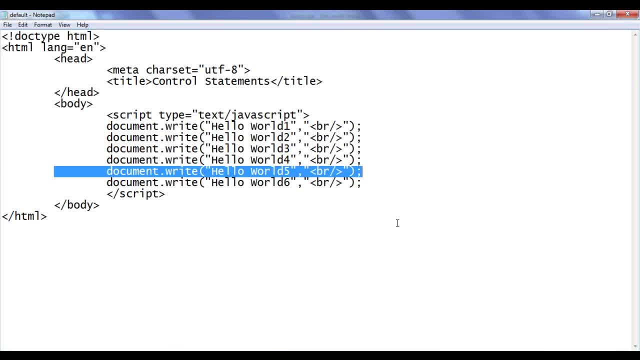 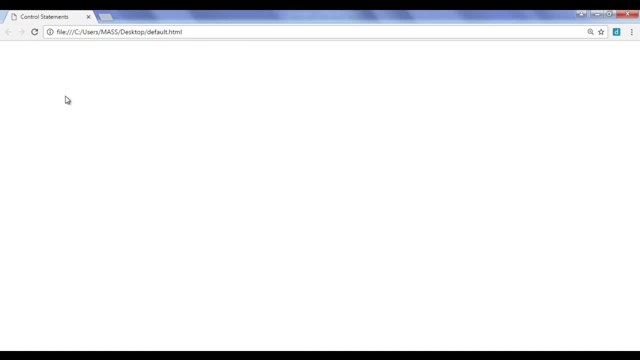 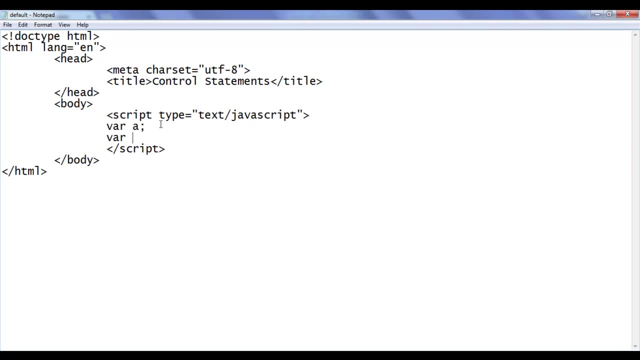 statement. Let me explain clearly. I go to notepad, I select these lines of code say: delete file, save. go to browser and refresh. We don't have any output Now. in between the script tag, I say: var a semicolon, var b semicolon, var c semicolon. 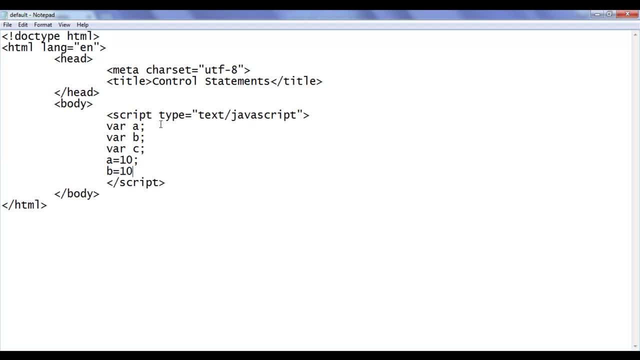 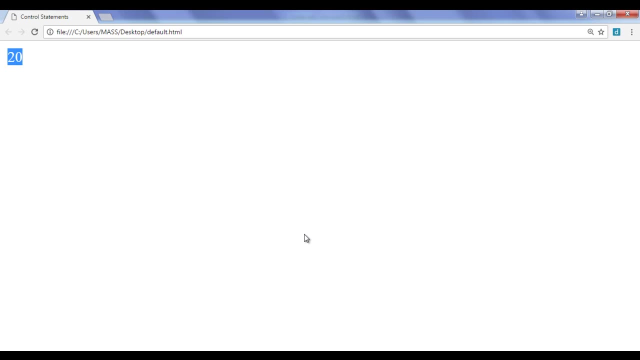 a equal to 10, semicolon b equal to 10. semicolon c equal to a plus b semicolon. then documentwrite display the value of c semicolon file save. go to browser and refresh. we got the output 20.. 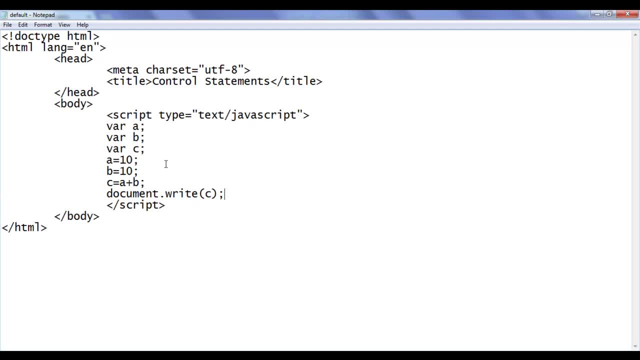 So what browser is doing here? Browser is executing each of these statements top to down, sequentially, one after the another, and displaying the value of c on the screen. First it creates a variable a, then it moves to the next statement. creates a variable. 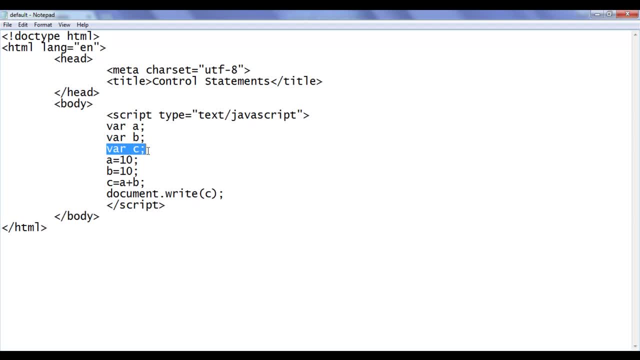 b. then it moves to the next statement. creates a variable c. then it moves to the next statement. puts the 10 in a. then it moves to the next statement. puts the 10 in b, then it takes the value of a. 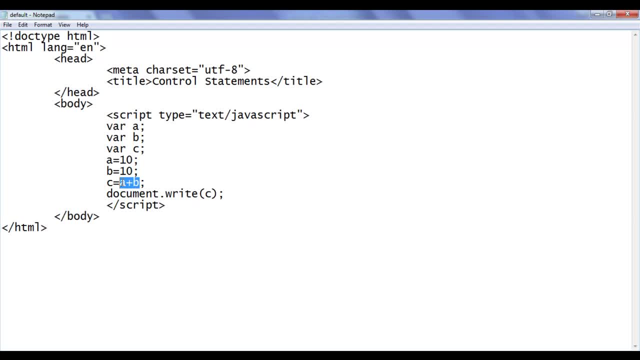 value of b adds them together, 20.. 20- it puts in c. Then it displays the value of c. We are getting 20 on the screen. You can see that no statement is skipped here. After executing this statement, the browser is moving to the next statement. So there is no break in the flow of execution of. 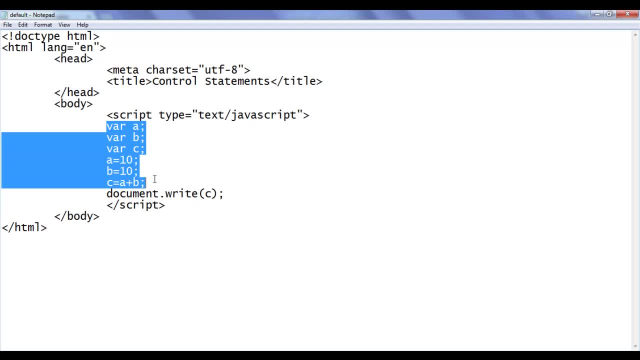 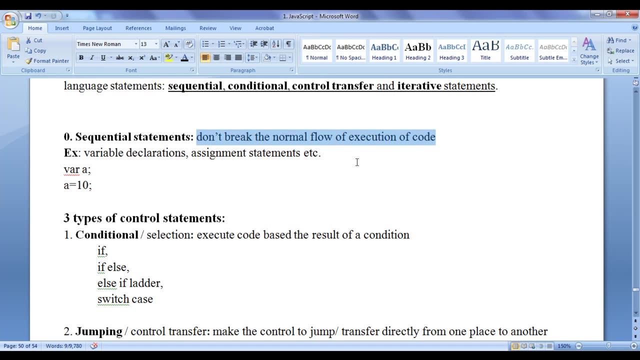 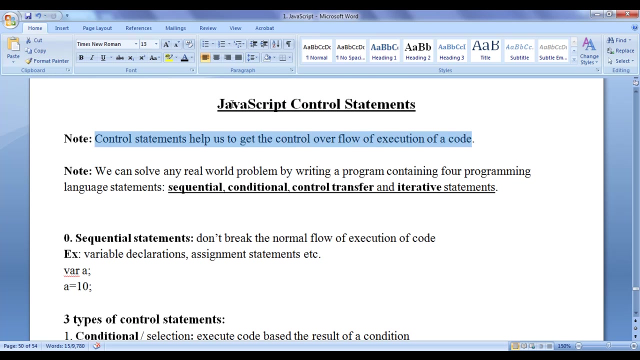 code Right. All statements are getting executed sequentially. Any statement which don't break the normal flow of execution of code is called as sequential statement. Hope you guys have clearly understood. Sequential statements don't break the normal flow of execution of code. As I told, to get the control over flow of execution of code we take help of JavaScript. 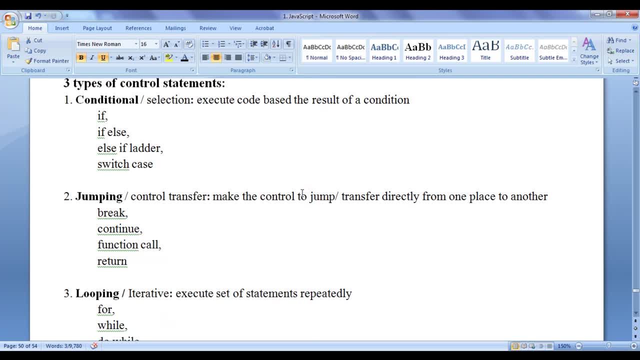 control statements. There are three different types of control statements provided by JavaScript. They are conditional statements, jumping statements, looping statements. Conditional statements are also called as selection statements. Jumping statements are also called as control transfer statements. Looping statements are also called. 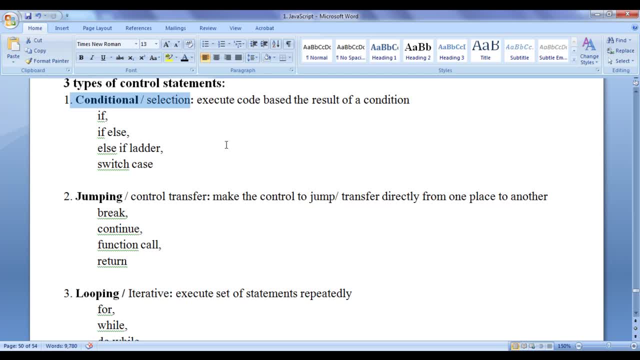 as iterative statements, Conditional statements or selection statements. execute the code based on the result of a condition. That means you can select some set of statements and execute them based on the condition. If the condition evaluates to true, execute those set of statements. Otherwise, do not execute. 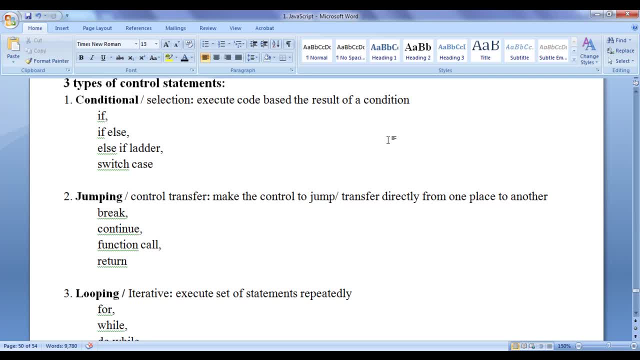 Right. Conditional statements help you to execute a statement or set of statements based on the result of condition. If the condition evaluates to true, execute some set of statements. Else, execute some other set of statements like that If, if else else, if ladder switch case are, 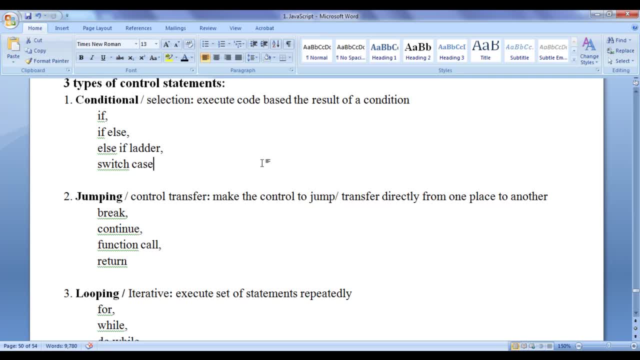 considered as conditional or set of statements. If, if else else, if ladder switch case are considered as conditional, throws on you a chance on locking the root case set and jangan be careful. Jumping and control transfer statements: make the control to jump or transfer directly from one place. 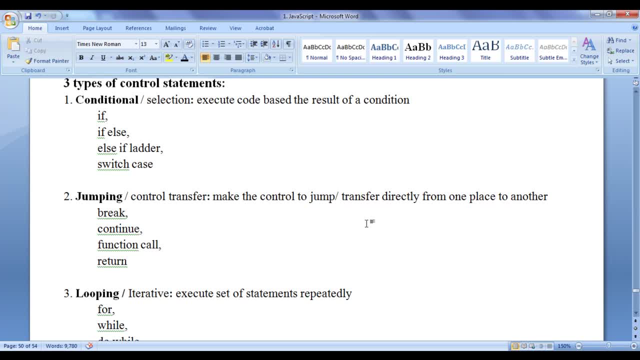 to another place. That means if we want to skip some set of statements and jump from one place to another place directly or transfer the control from one place to another place directly, we take help of jumping or control. transfer statements, Break, continue, functionalist. cell controlщее statement are some, And between jump and control transfer statements we also have choices that are optional Selection statements. Otherwise those are not available here. If you want to skip and control the control statement, you can switch the controls directly from one place to another place directly. We take help of jumping or control transfer statements. alkal dis. 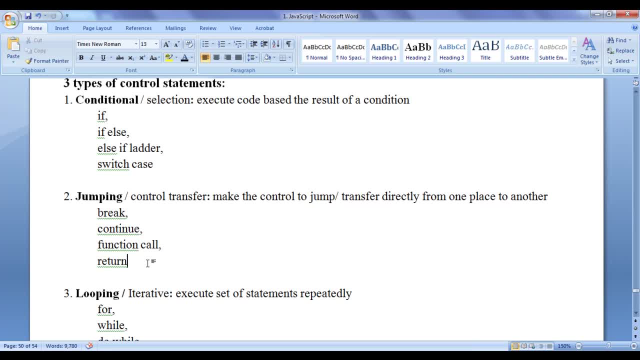 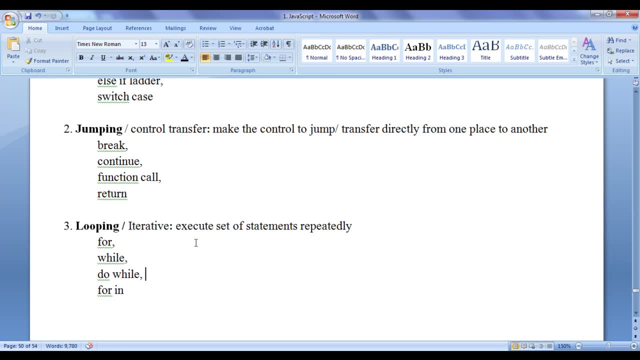 function calls return statements are considered as jumping or control transfer statements. Similarly, looping or iterative statements execute set of statements repeatedly. That means if we want to execute a single statement or set of statements repeatedly, we take help of looping or iterative statements For loop while loop, do while loop for in loop.